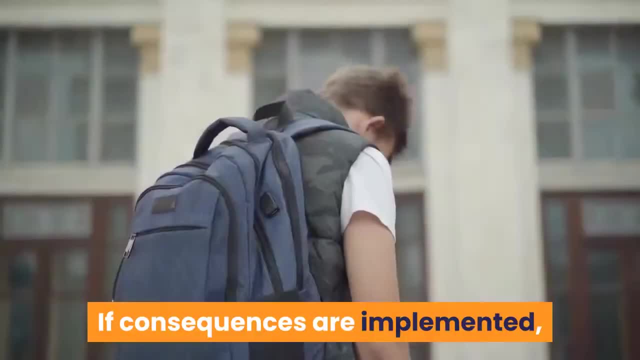 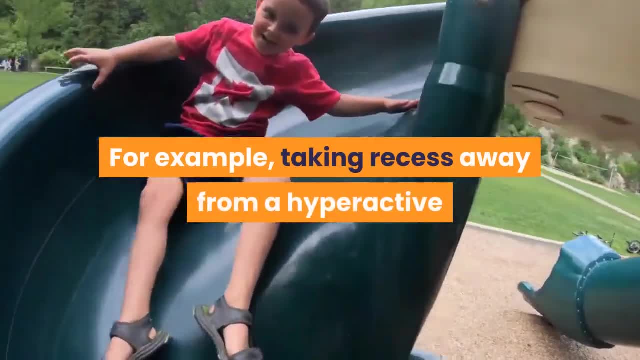 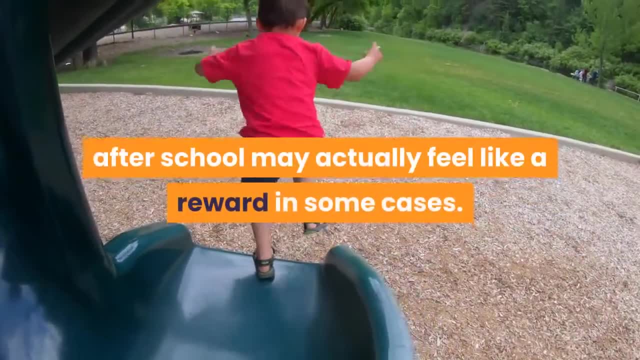 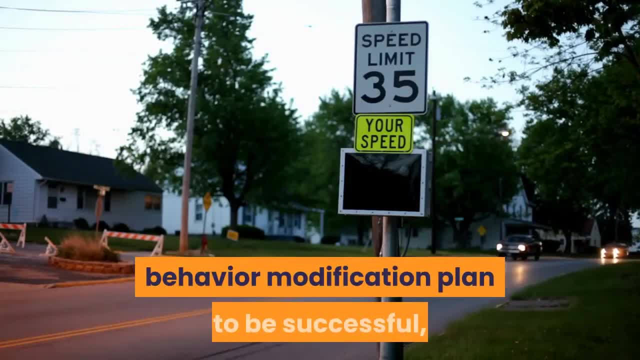 If consequences are implemented, they must be carefully selected to be a disincentive to the child. If consequences are implemented, they must be carefully selected to be a disincentive to the child. plan to be successful, it must be consistently enforced. Rewards and consequences should. 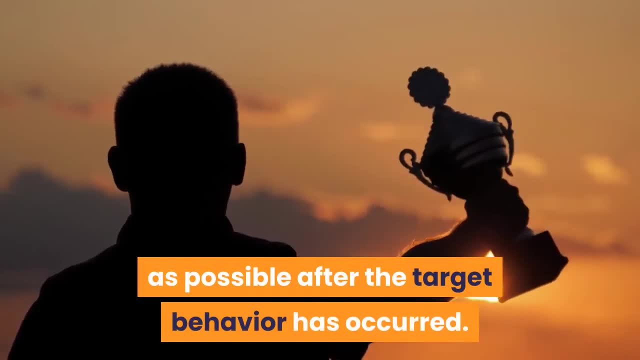 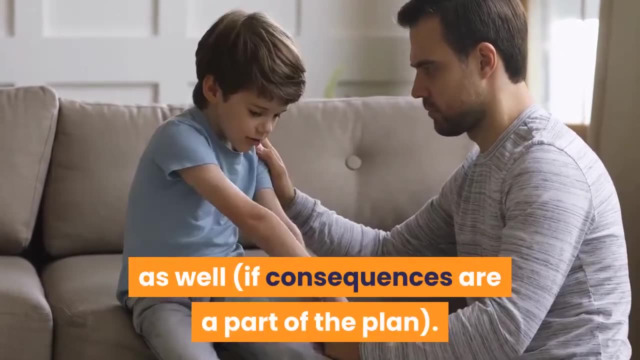 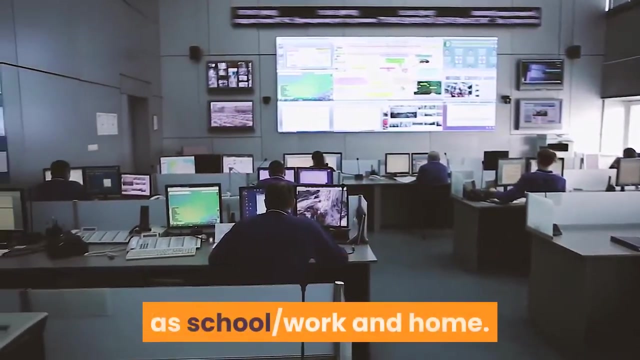 be given as soon as possible after the target behavior has occurred. Negative behaviors must receive consequences immediately as well. if consequences are a part of the plan, Frequent monitoring and feedback are also helpful, as is implementing the plan across settings such as school work and home Behavioral interventions for adults. Adults can also benefit. 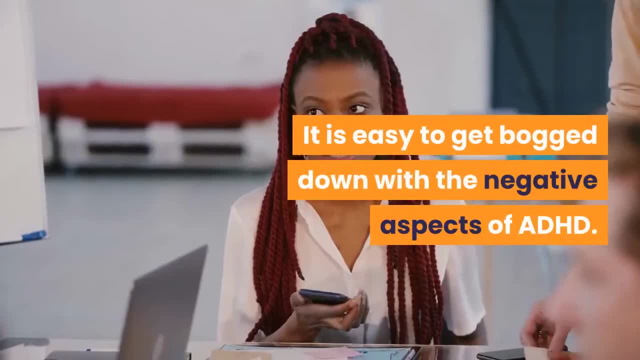 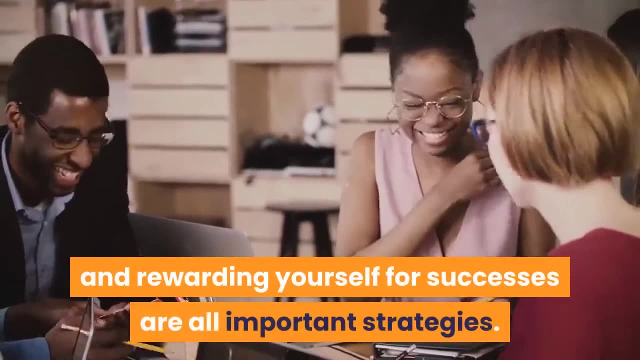 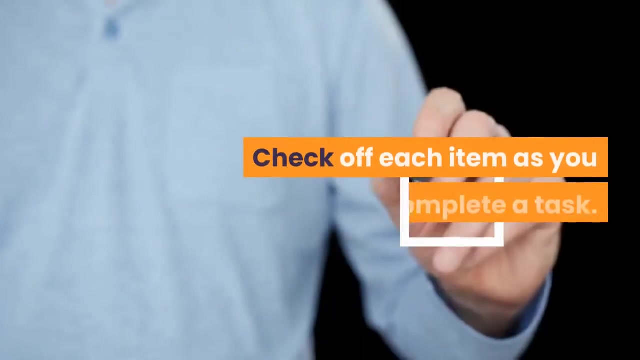 from a reward system, It is easy to get bogged down with the negative aspects of ADHD. Encouragement, focusing on the positive and rewarding yourself for successes are all important strategies. Use lists to help keep yourself focused and on track. Check off each item as you complete. 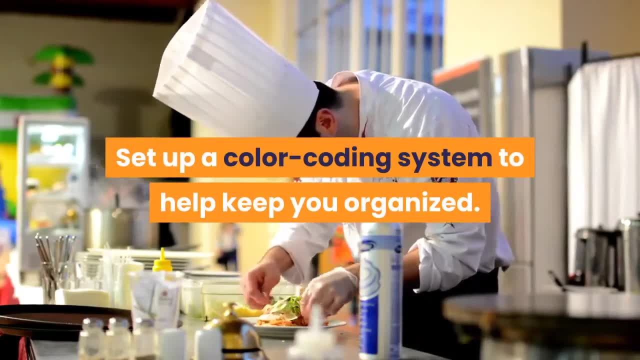 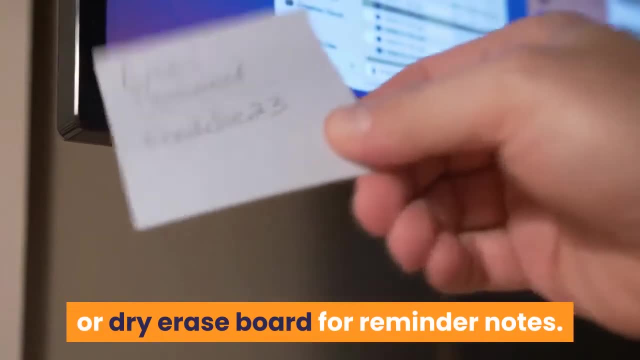 a task. Set up a color-coding system to help keep you organized. Use a daily schedule or planner. use post-its or dry erase board for reminder notes. No matter what your plan is, you must be focused on the positive aspects of the plan. If you 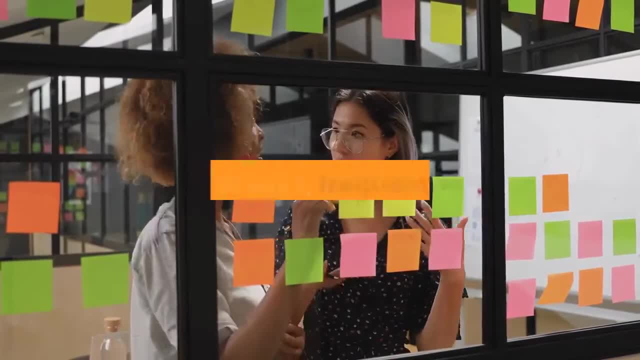 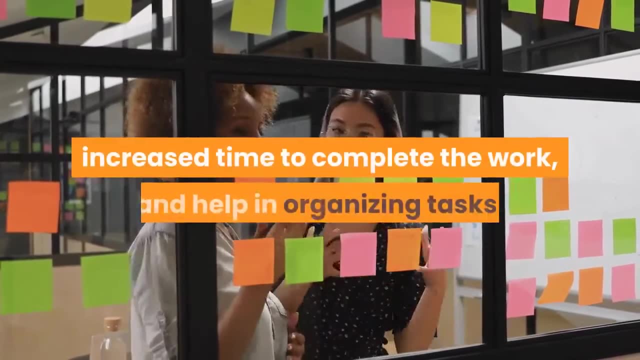 don't know what age. people with ADHD can benefit from regularly scheduled breaks, frequent feedback, work given in small increments reduce clutter and distractions, increase time to complete the work and help in organizing tasks. These are all ways to have an influence. 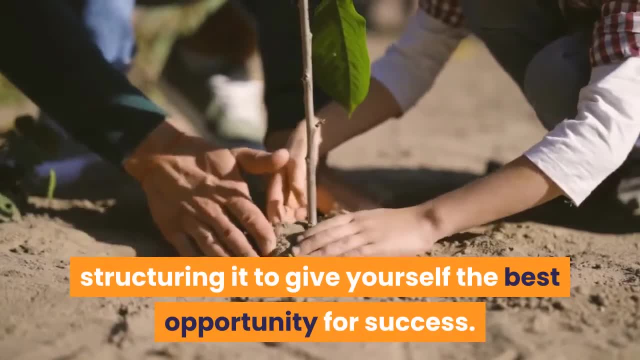 on your environment, structuring it to give yourself the best opportunity for success. 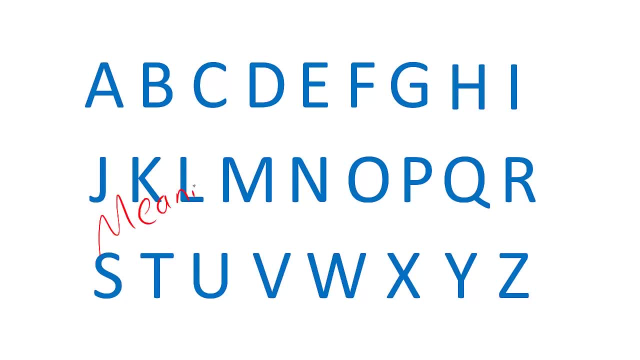 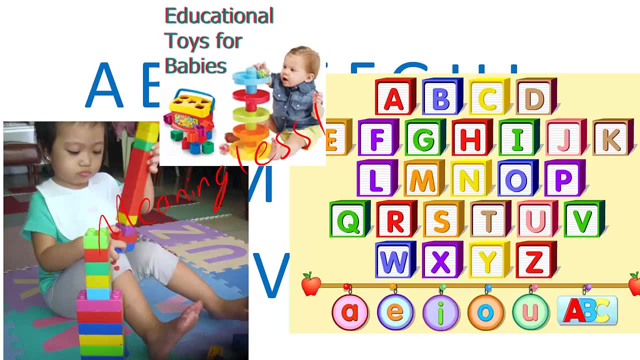 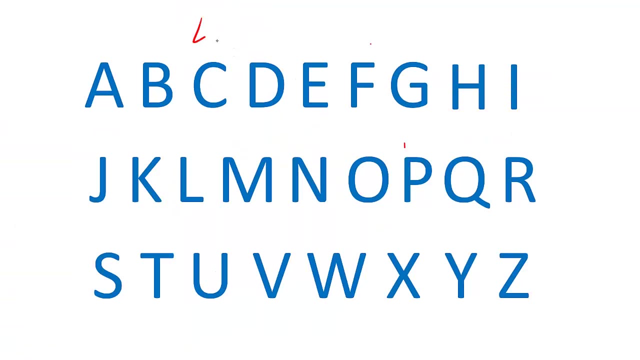 We use inherently meaningless symbols to communicate every day, Although you've probably seen these symbols since you were, before you even knew what they were. these symbols don't have any meaning, But we have developed a code called the English language that assigns meaning to these symbols.